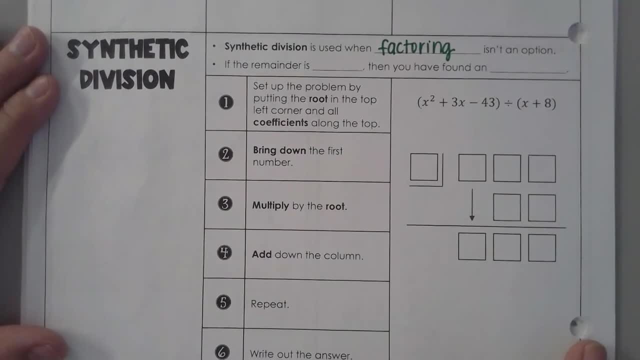 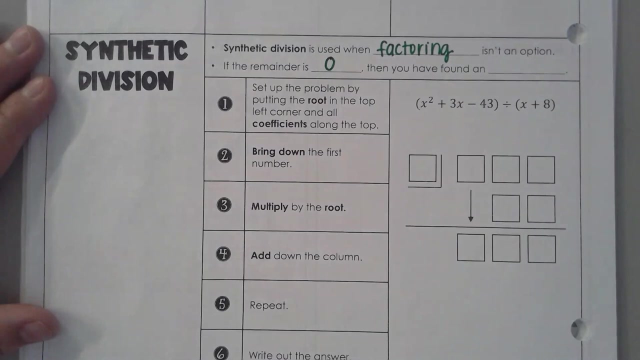 we're doing Now: synthetic division. it's a process. You've got to memorize the steps, but once you memorize them you can do them really quick. So if the remainder is 0, then you have found an x-intercept. 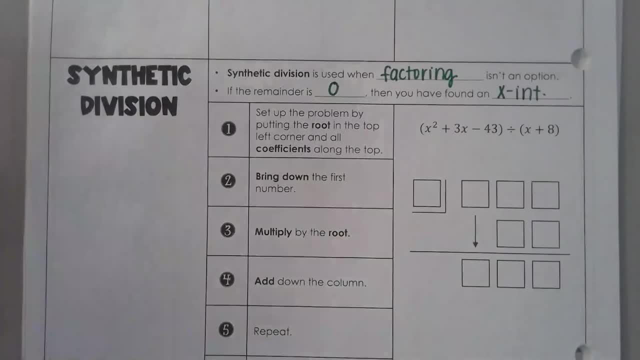 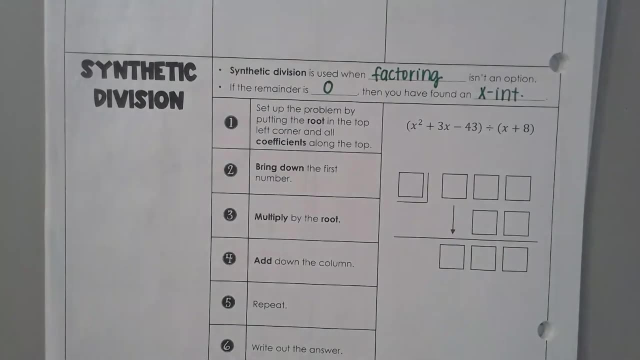 Normally we would do some more with this in another lesson, but we are skipping that right now, So you don't have to worry about that too much. So synthetic division. first of all, you have to set up the problem, So you've got to fill in some numbers. I've drawn boxes on this first one to guide you. 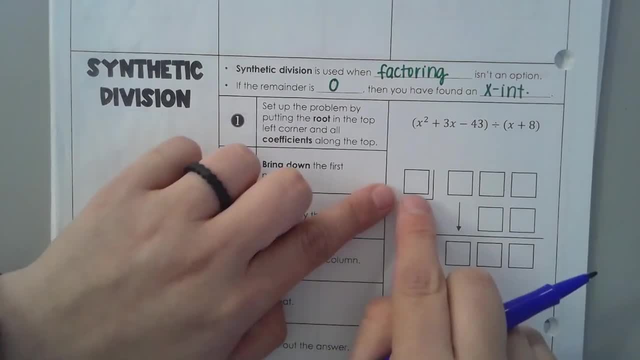 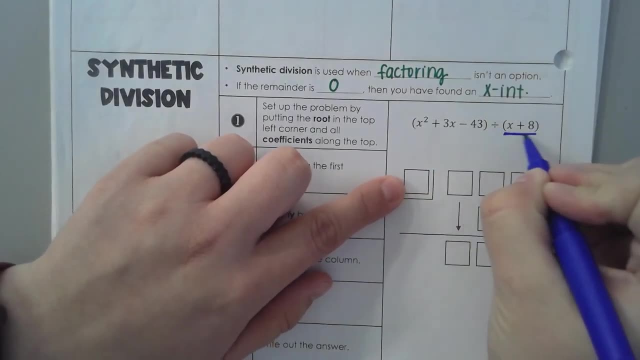 You won't always have those boxes. You'll just write in some numbers. So in the top left corner you're going to have like a little a number and that number is going to be the opposite of whatever you're dividing by. 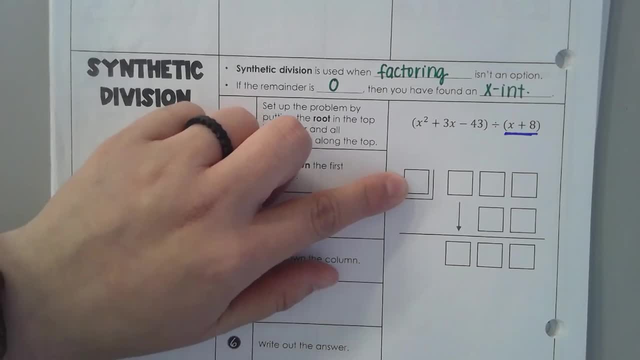 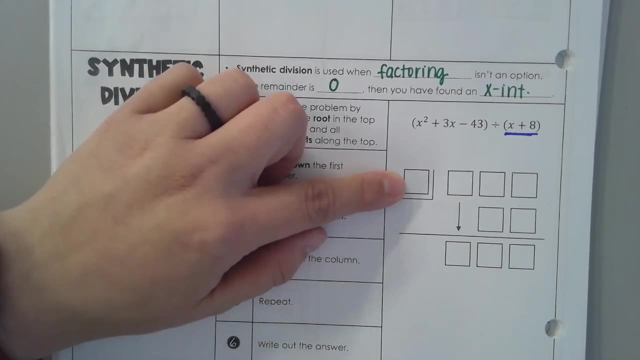 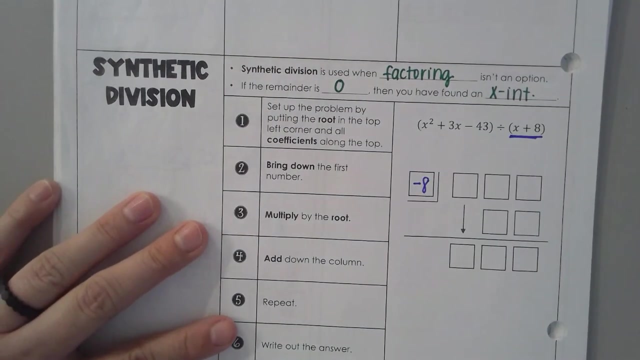 So we're dividing by x plus 8.. It's basically like I'm setting that equal to 0. If I set that equal to 0, I would get x equals what Negative 8.. So that's the number that goes in the top left corner. 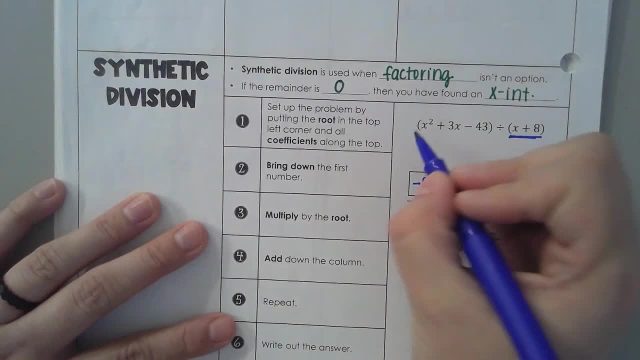 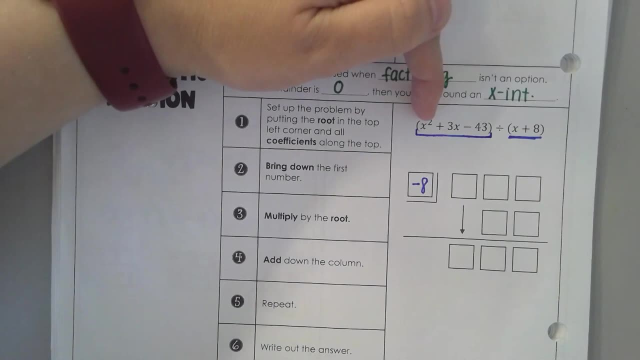 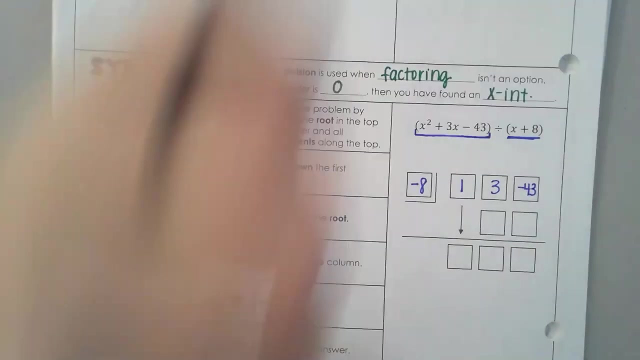 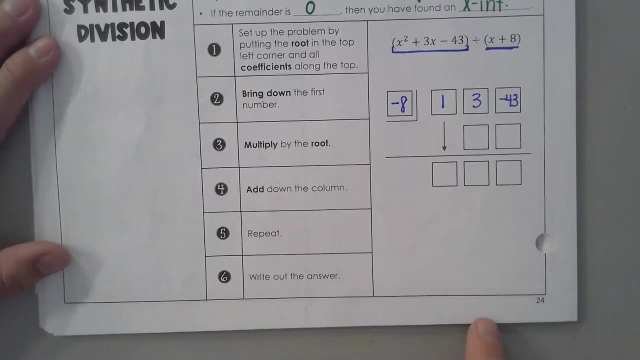 And then you're going to fill in your coefficients. Okay, To your first polynomial. So the numbers in the front. So, technically, what's in front of the x squared, 1.. 1,, 3, and then a negative 43.. 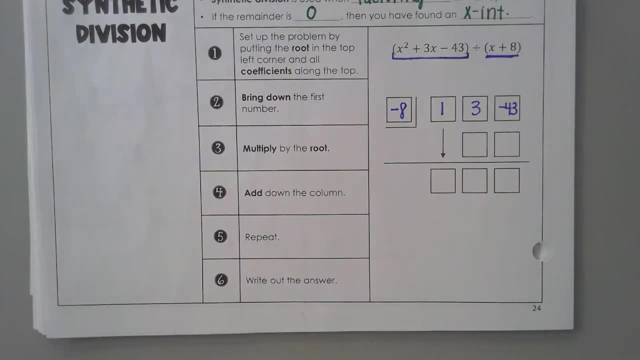 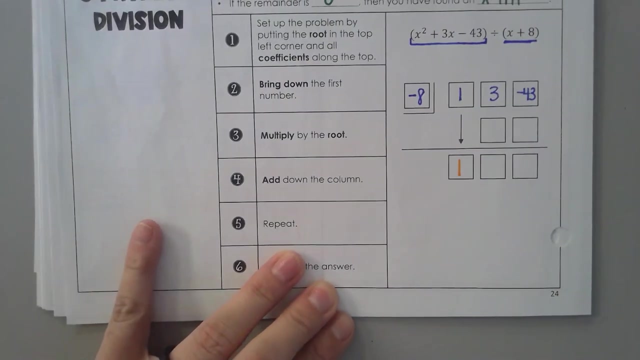 And from here on out it's: bring down, multiply, add, multiply, add, multiply, add. So you bring down the first, this first number where I drew an arrow. Bring down the 1. And then we multiply this number times our corner number, So our negative 8.. So what's 1 times? 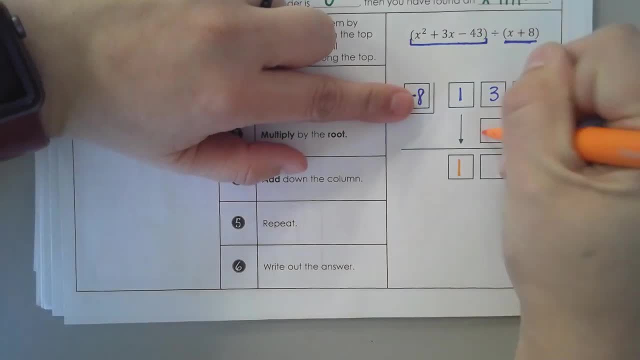 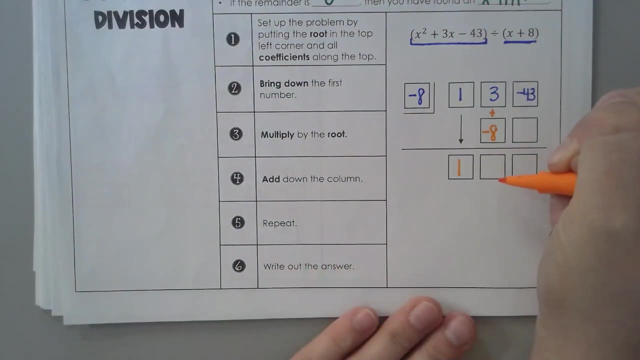 negative 8? Negative 8. Yep, And that goes here. So we multiplied and then we add straight down 3 plus negative 8. is what? Negative 3. Mm-hmm. Negative 3. Mm-hmm. 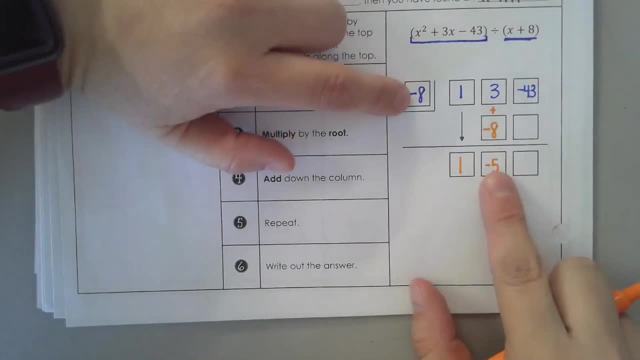 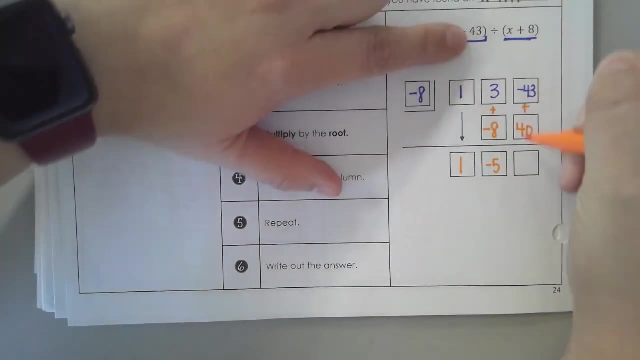 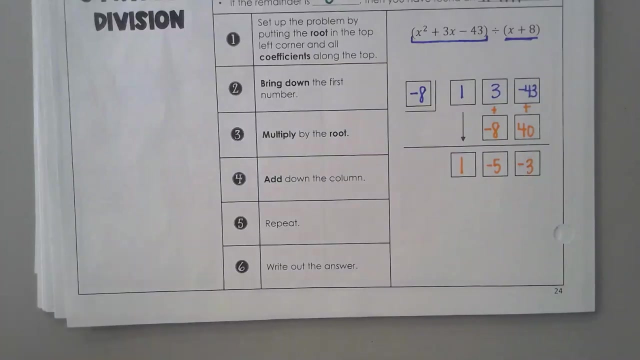 Now we multiply Negative 8 times negative 5 is 40.. 40. And then we add straight down and we get what? Negative 3. Negative 3. These new numbers tell us like the coefficients of our answer. So here's. 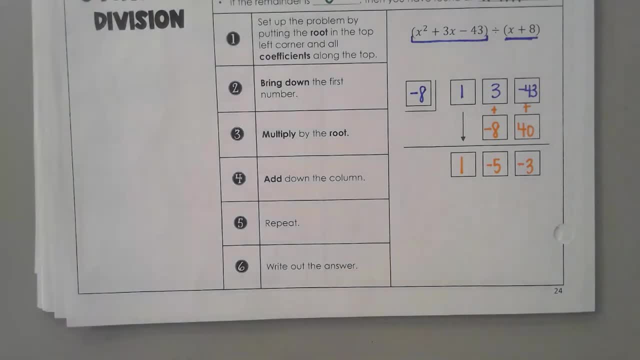 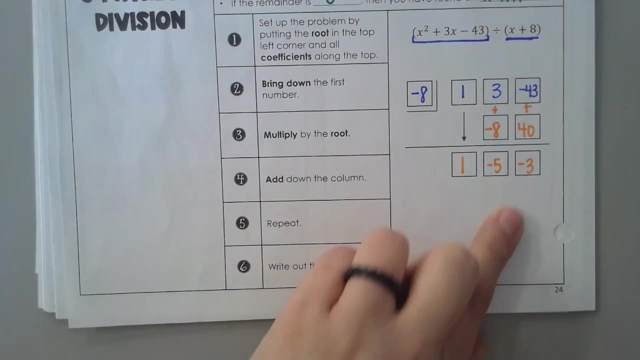 what I want you to do. You're going to start. we're going to start on the far right and work our way over The far right number, the negative 3, that is going to be our remainder, The next number in line, that is just going to be a plain number, which is we call a constant. 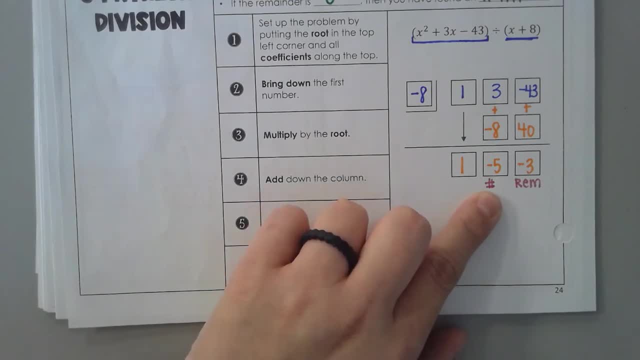 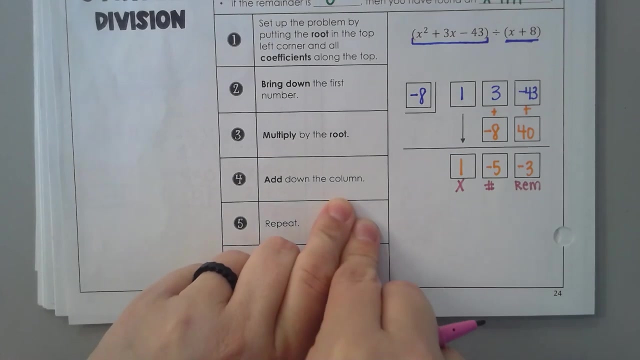 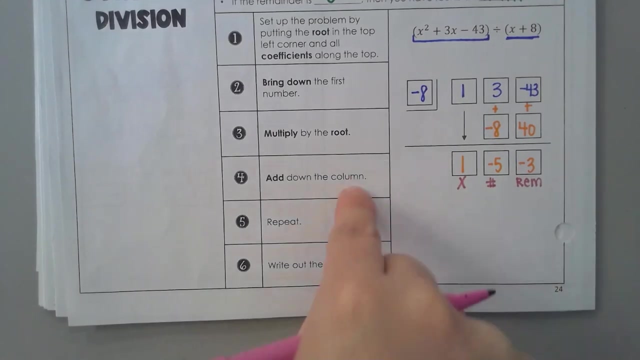 The next number over is going to get an x with it. If I had more numbers, the next one would get x squared, the next one would get x cubed, and so on, But it's always remainder number or constant: x, x squared, x cubed, x to the fourth, as many as you've got, And 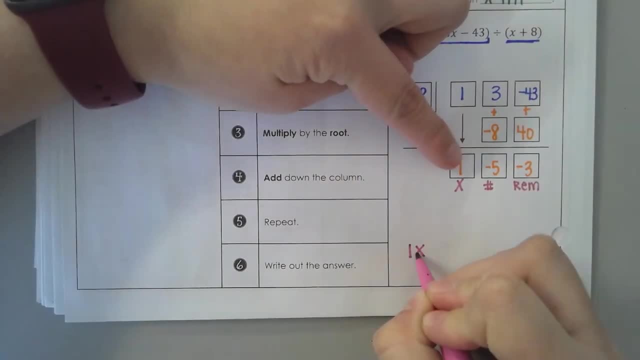 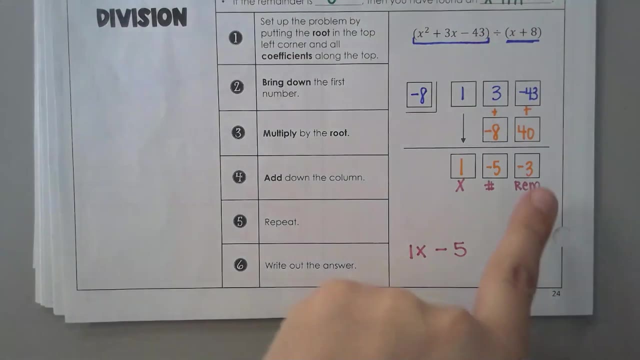 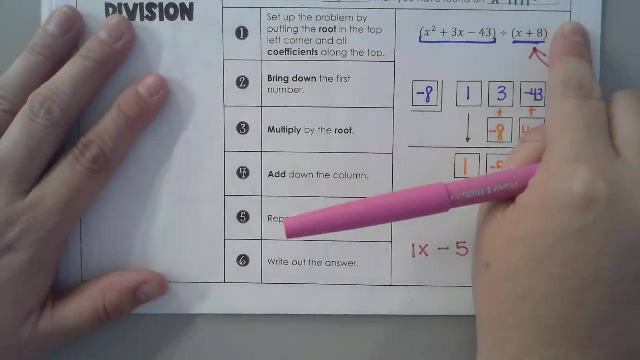 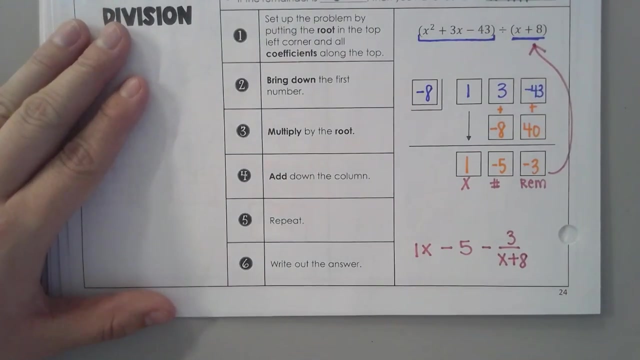 so we can write our answer as 1. 1. 1. 1x minus 5, and then our remainder always goes on top of what we were dividing by. So it's going to be minus 3 over x plus 8.. So it is a lot. it is a process, but once you 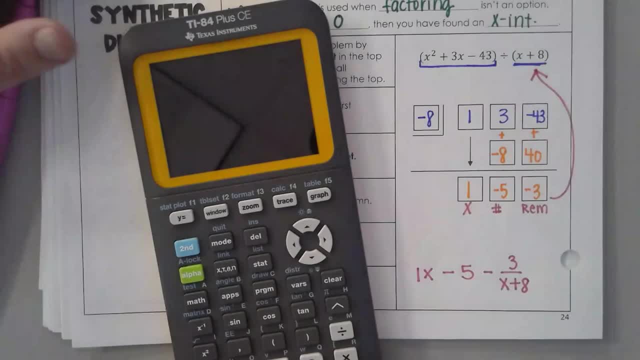 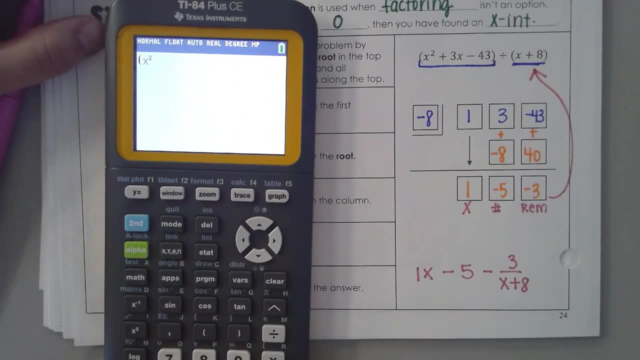 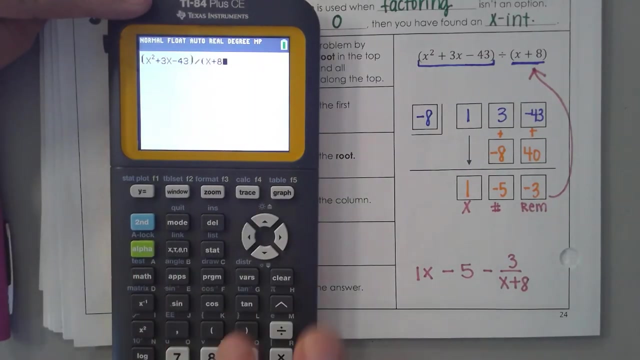 get that pattern kind of memorized. you can do them pretty quick And I'm going to show you how you can do them in the calculator. x squared or check it in your calculator. I guess 3 divided by x plus 8. I get that. 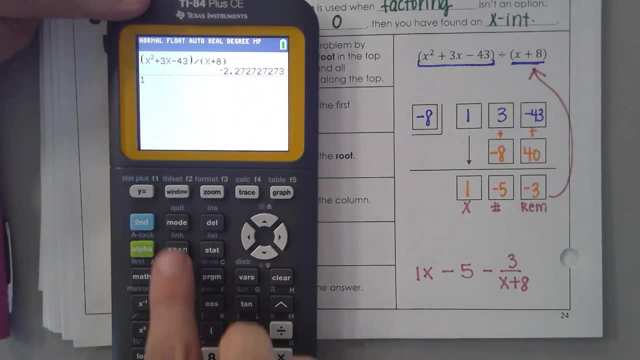 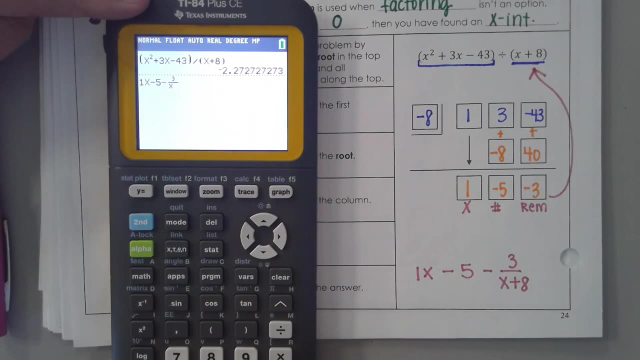 And then I'm going to check my answer: 1x minus 5 minus 3 over x plus 8.. Do they match? Yeah, Yep, they do. So I did it right. So we're going to do some more examples. 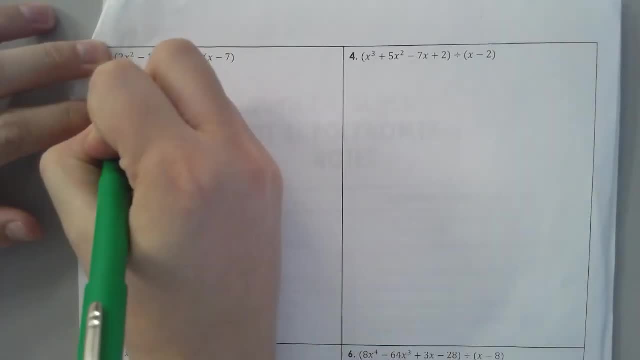 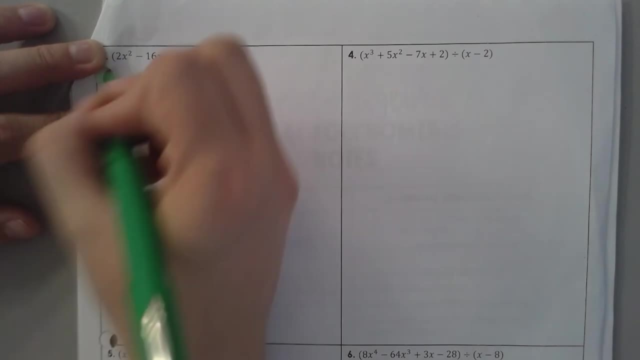 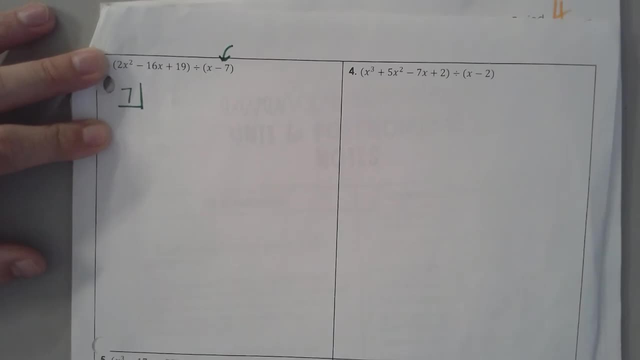 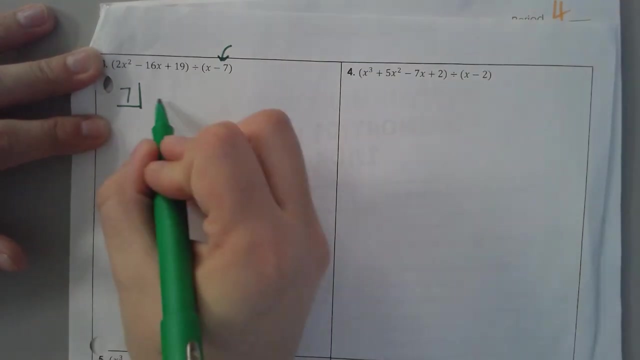 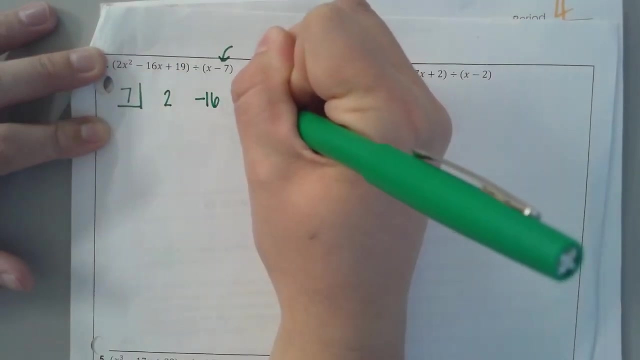 Positive 7.. Positive 7. going to be the opposite of that number. So I'm dividing by x minus 7.. You're going to put a positive 7 in the box And then what numbers go across the top? Yep 2,. negative 16, and 19.. Leave a space and draw a line. 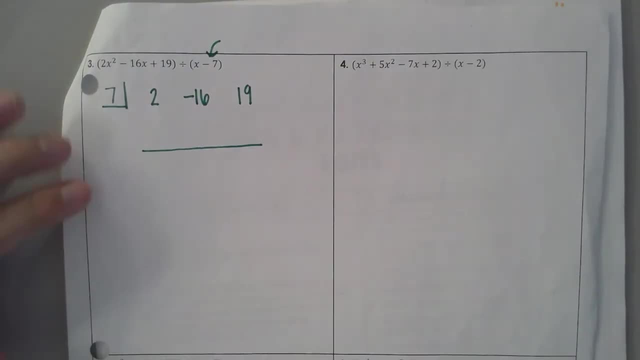 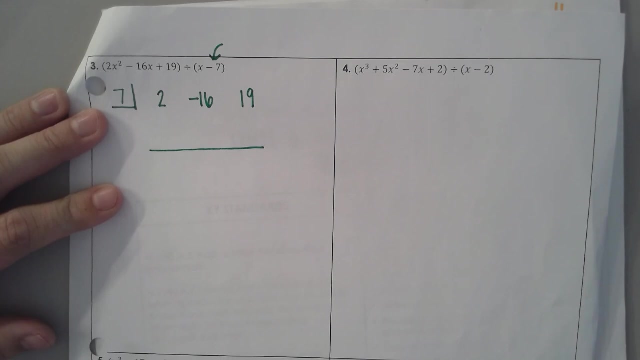 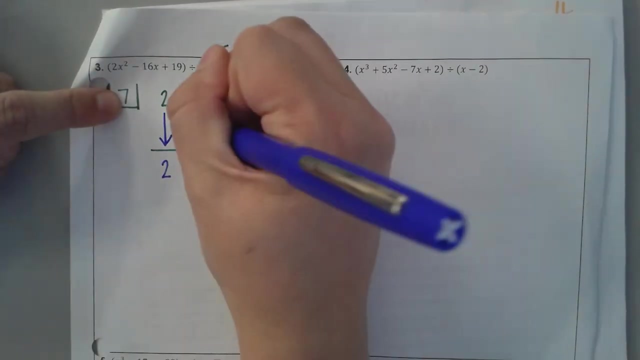 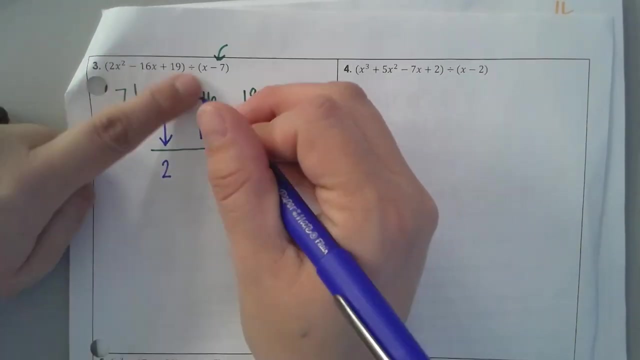 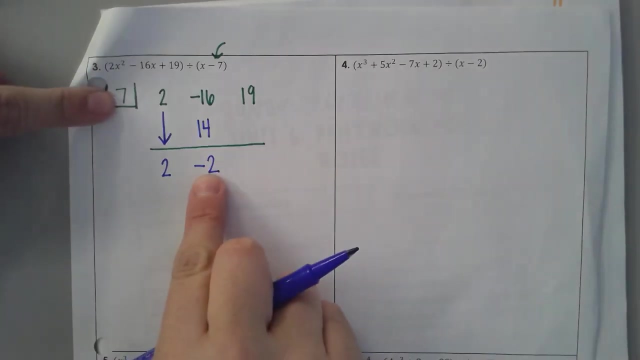 So what's my first step? Not yet Bring down the first number. So I bring down the 2, and then I multiply: 2 times 7 is 14.. And then you add: What do I get when I add Negative 2.. And then you multiply, And what do I get? 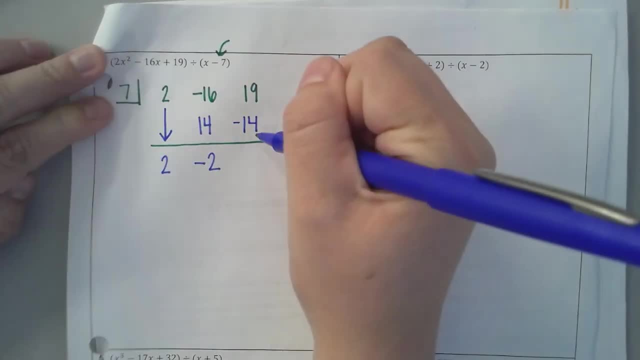 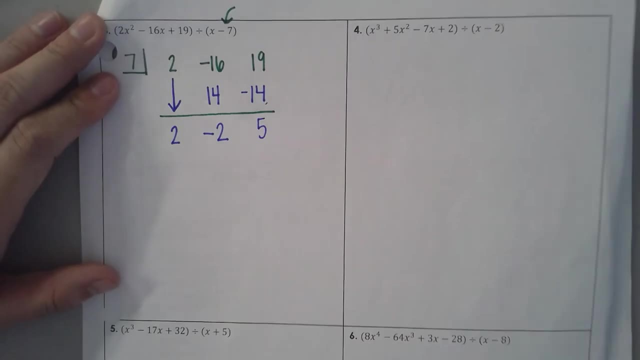 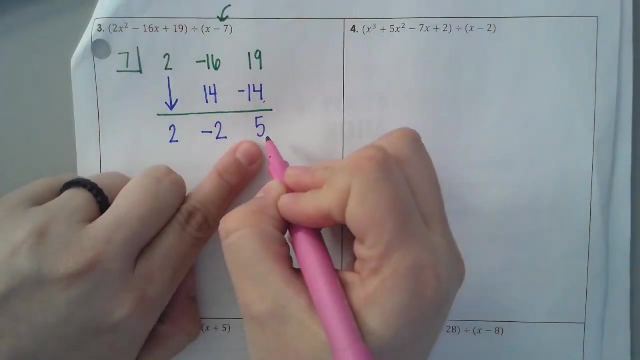 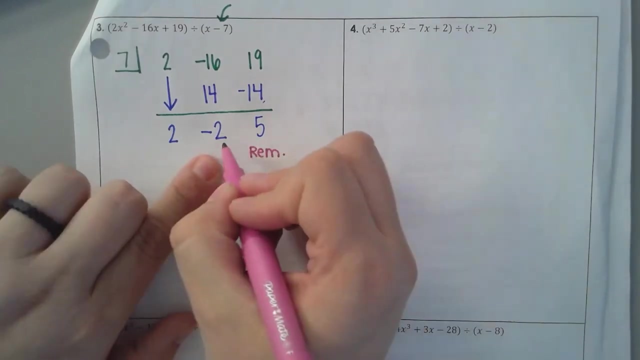 Negative 14.. And then I add: to get what? 5.. So you're not done here. This is not your final answer. Start on the far right. 5 is my. what Remainder Negative 2 is going to be? it's my, it's just my plain. 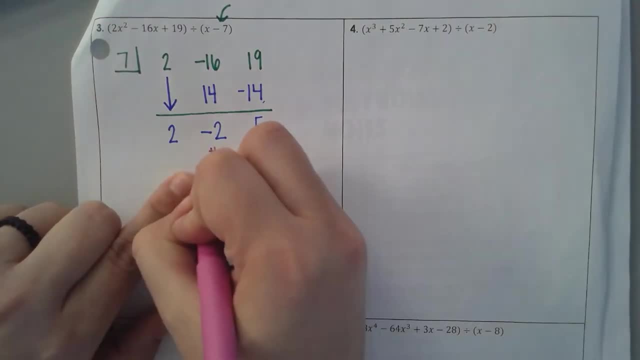 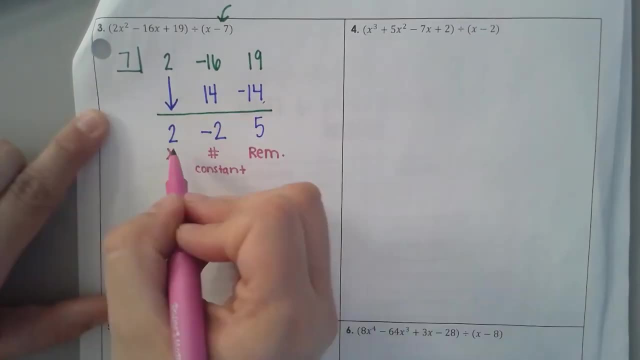 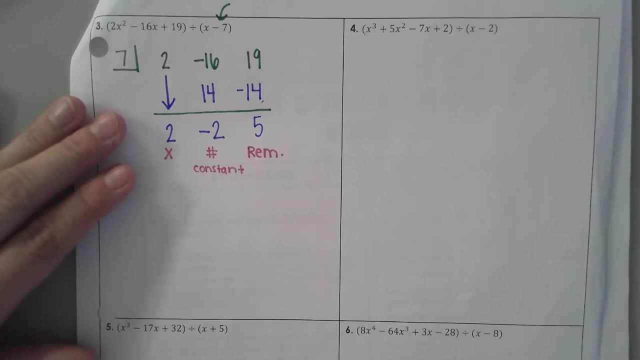 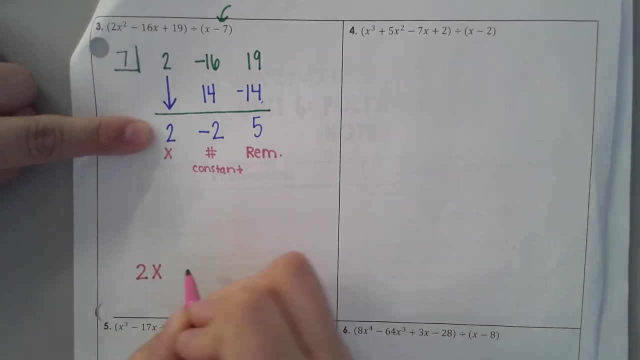 number, which is we call a constant, And then, from there on, I build up my x's, So this one gets an x. If I had another one, it would be x squared, x cubed, and so on. And so my final answer is 2x minus 2, just a plain number. And then what do I do? 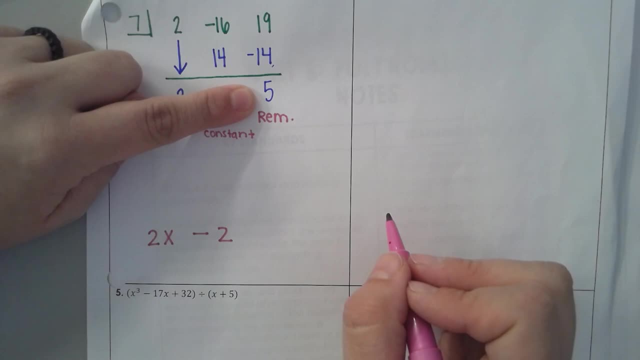 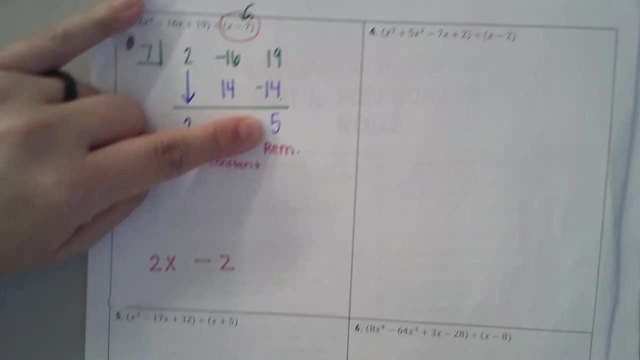 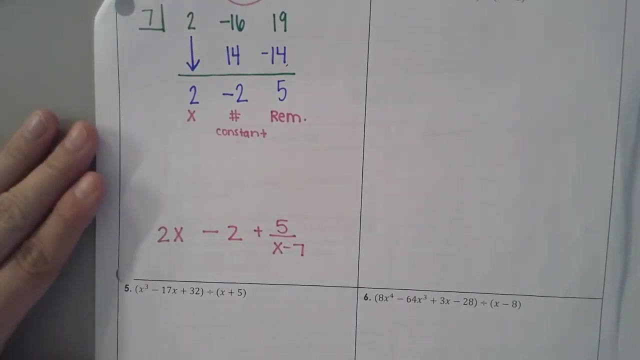 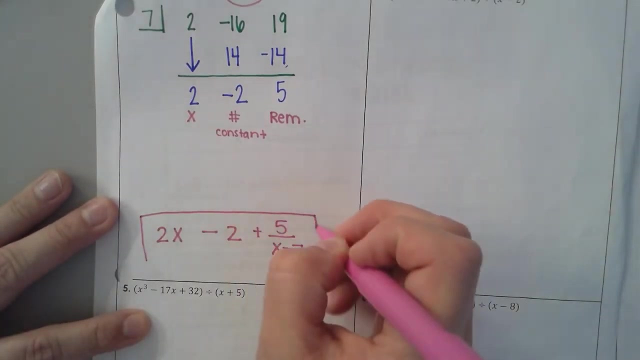 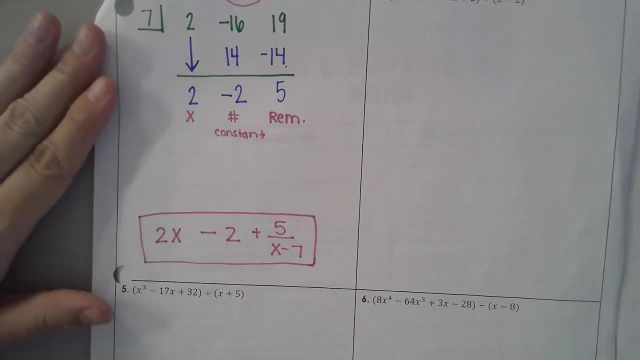 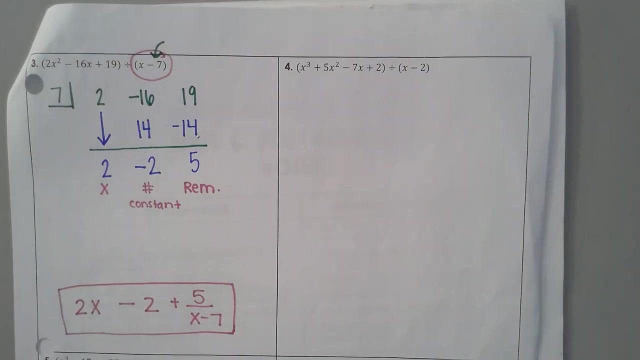 with my remainder. Yes, it goes 5 over x minus 7.. And that's your answer. So it stops when we're in a situation where we would then have to solve this equation? No, probably not All right number 4.. Set up your problem. 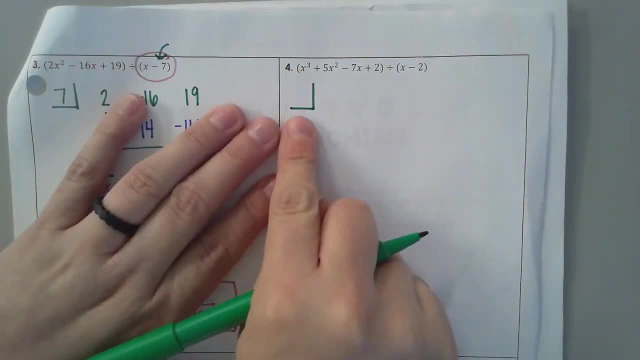 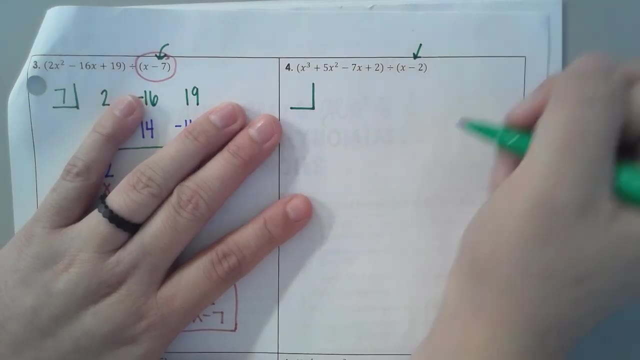 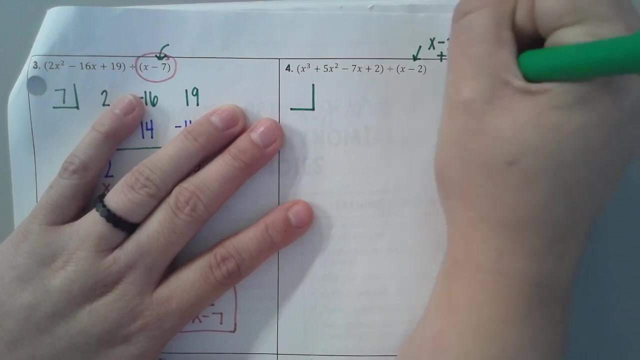 What number goes in this top box? Yep, you always take the opposite of that. So basically, really, what I'm doing is x minus 2 equals 0. If I add 2, I get x equals 2.. So a 2 is what goes in the top left box. 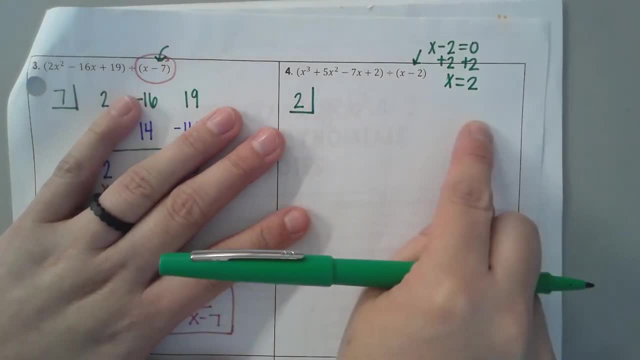 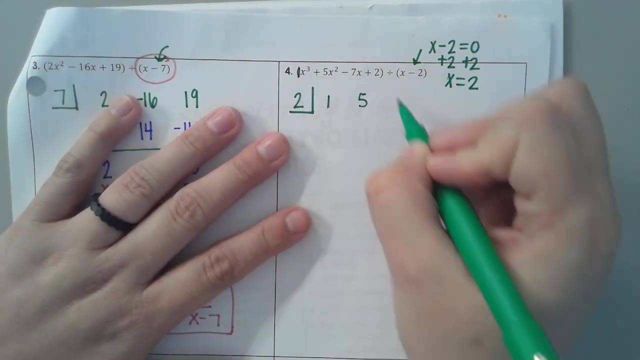 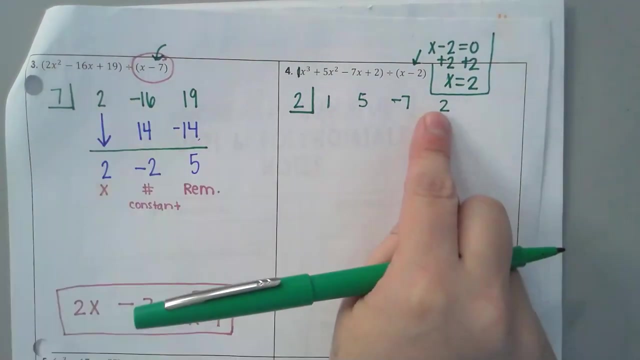 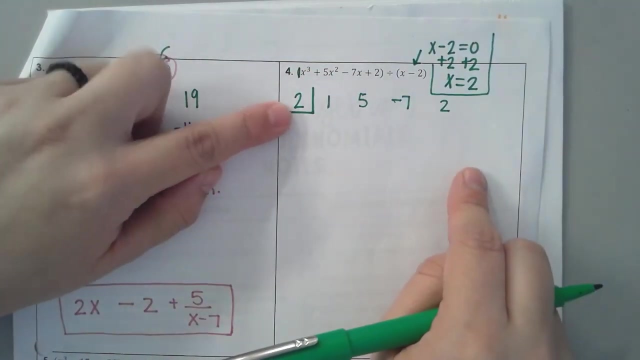 And then your coefficients, Which are 1,, 5, negative 7, and 2.. Those numbers go across the top. So for you that just came in, this is a method of dividing called synthetic division. It's a way to divide. 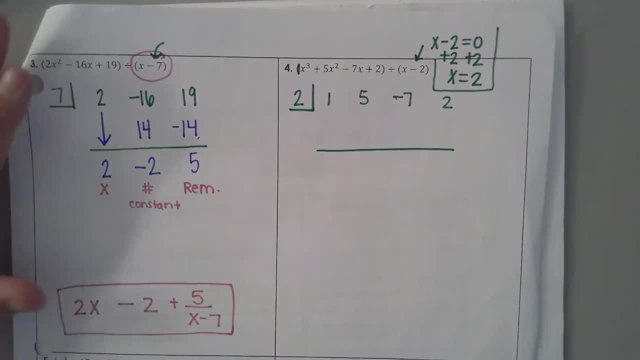 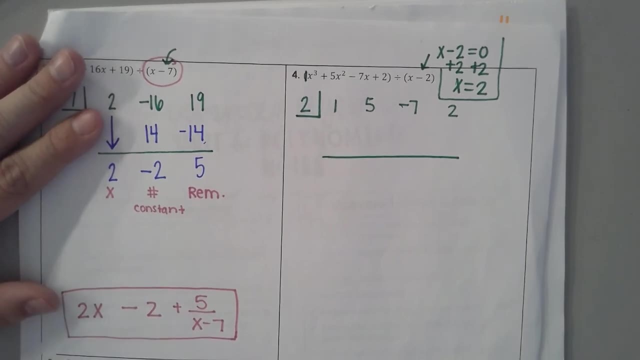 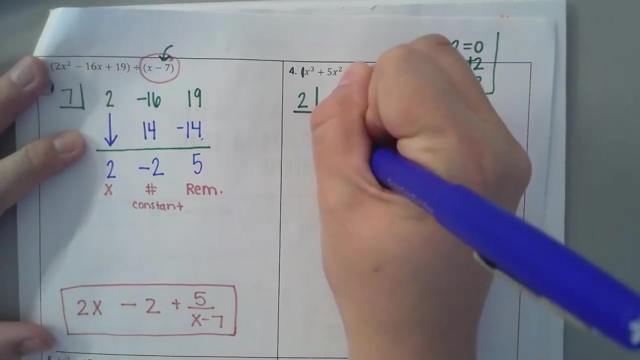 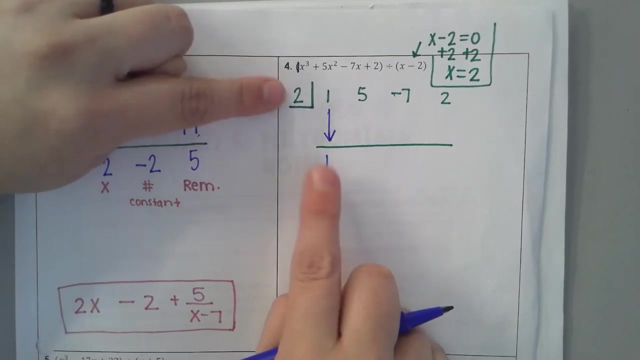 when you, when it doesn't divide evenly. There is another method. it's a long division. you'll learn that in mr Adams's class, but I just do synthetic division. so you always bring down your first number to bring down the one, and then you multiply two times. one is to add, so it's multiply, add, multiply. 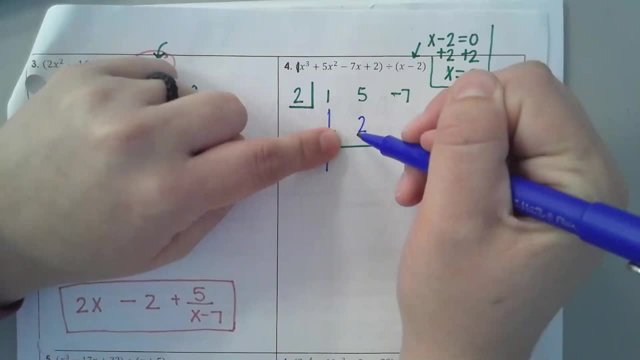 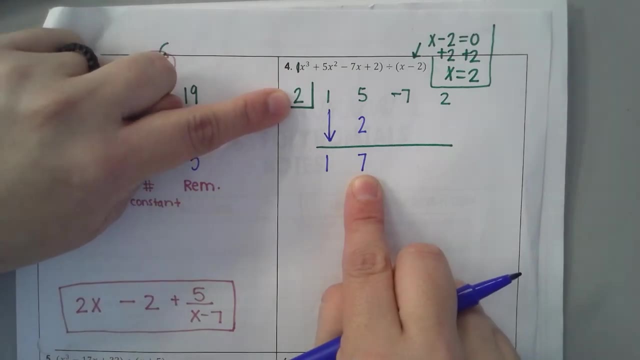 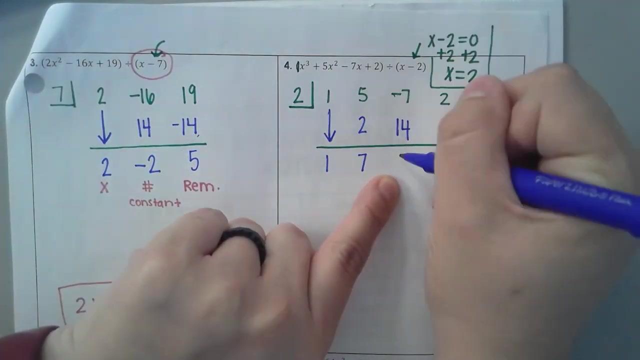 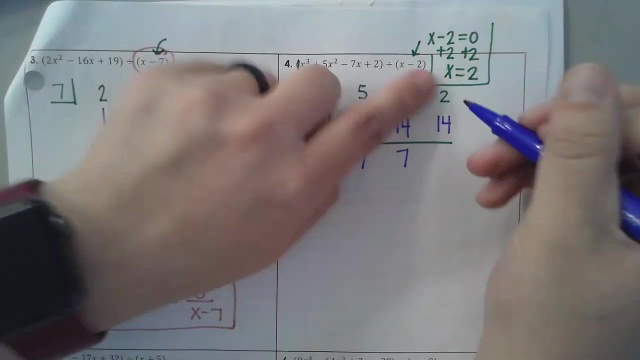 add, keep going. so what's five plus two? and that seven goes down there, and then I multiply that by the two to get 14, and then I add straight down to get seven, and then I multiply by the two to get 14 once again, and then I add to get 16. 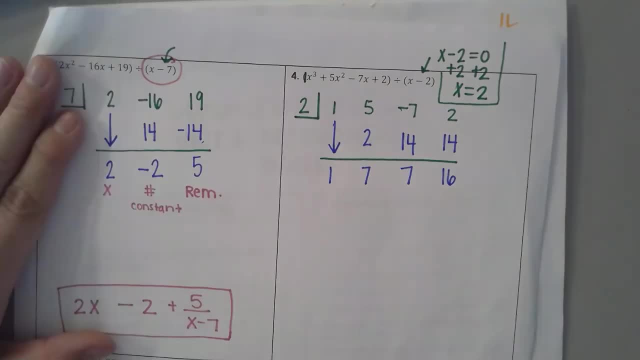 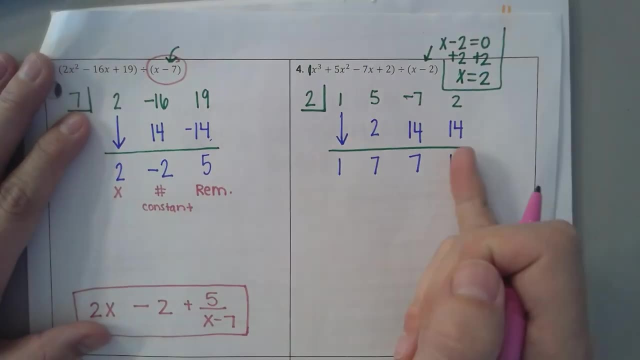 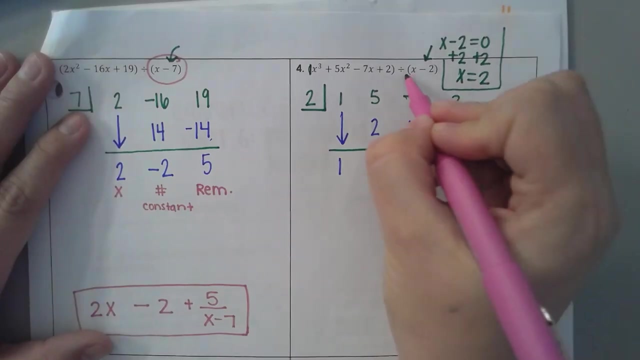 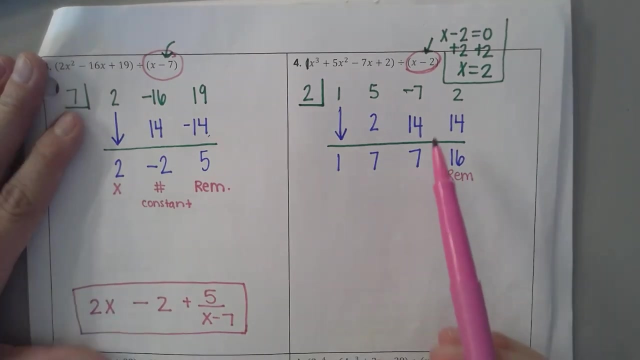 the number we go, we go backwards. the last, the 16, is your remainder, and you always put your remainder over in a fraction. what you were dividing by the next one is going to be your constant. so it's just a plain number. it does not get an X or anything. 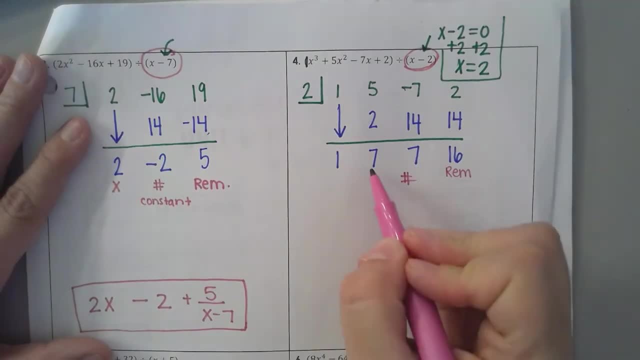 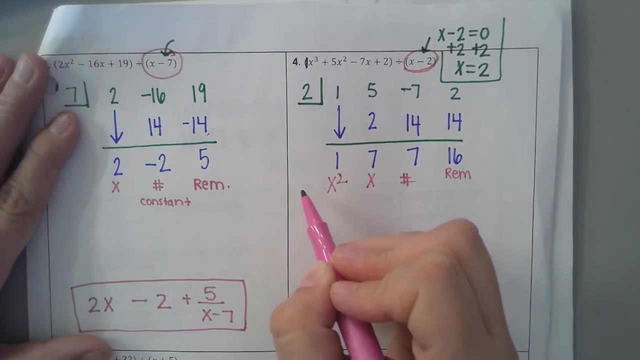 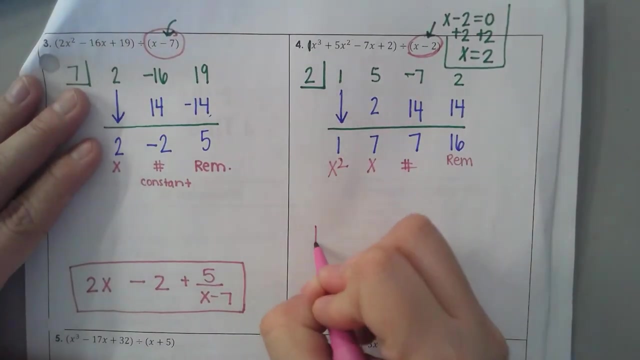 I just like to put a number into there. and then the next one gets an X, the next one gets an X squared. if I had another number, it would be an X cubed, and the next to the fourth, X to the fifth, so it's 1x squared. you don't have to put the one plus seven. 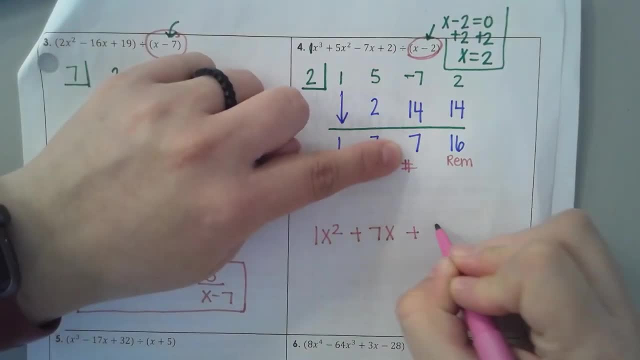 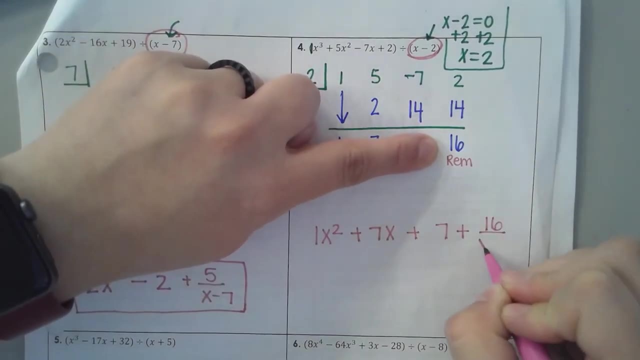 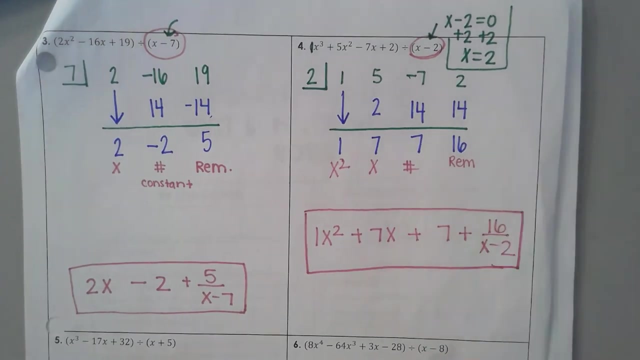 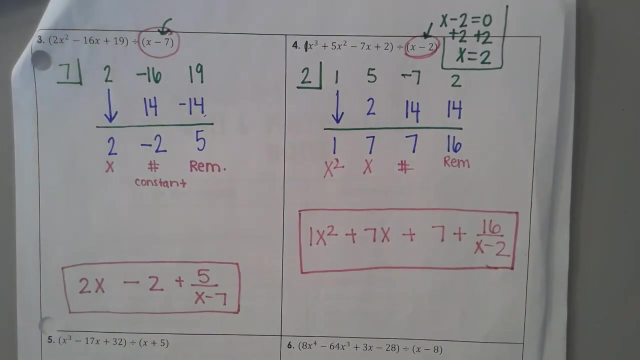 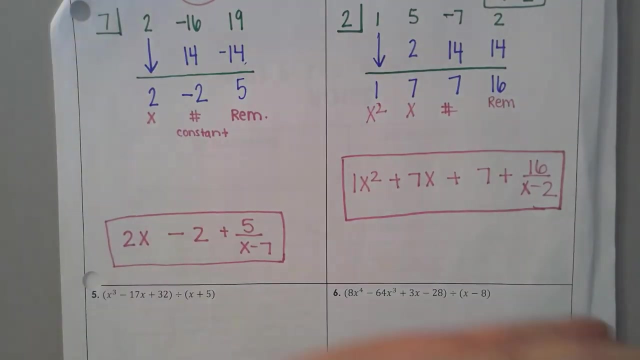 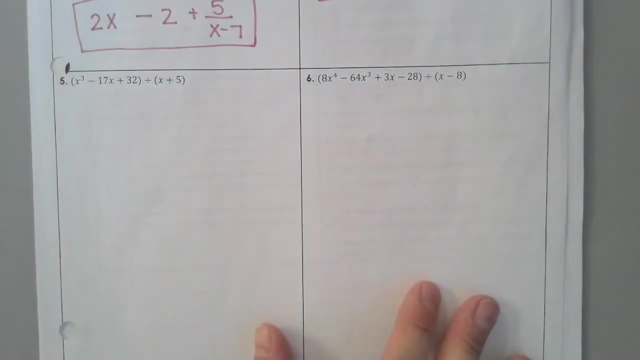 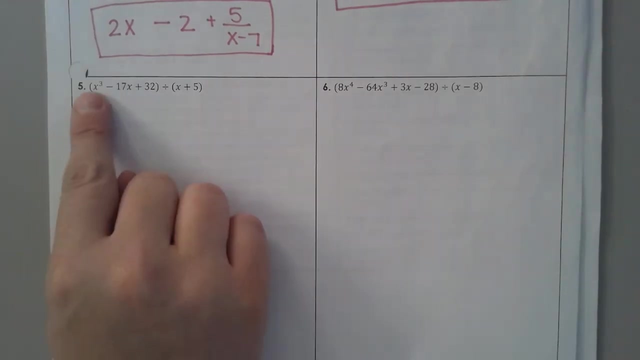 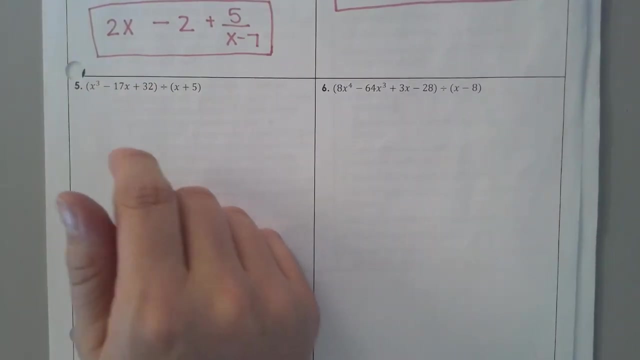 X plus seven, just a plain number, and then my remainder is over X minus two. now, before you get to going too far ahead on number five, there's something that's a little different about that one. so are there any questions? so far? Number five, the one thing that will cause you to mess up. the only like tricky part of this is you need to make sure that you have all terms: one that are in order and two that you're not missing anything. 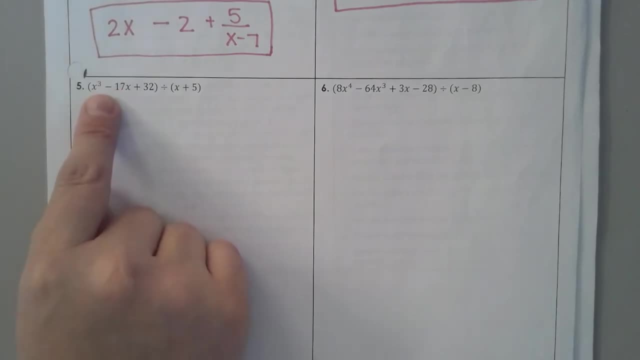 Notice on number five, I'm actually missing an x squared, So I went from x cubed down to x. If you are missing one of those terms, you have to put a zero in its place. So when we do our setup, what goes in the box? 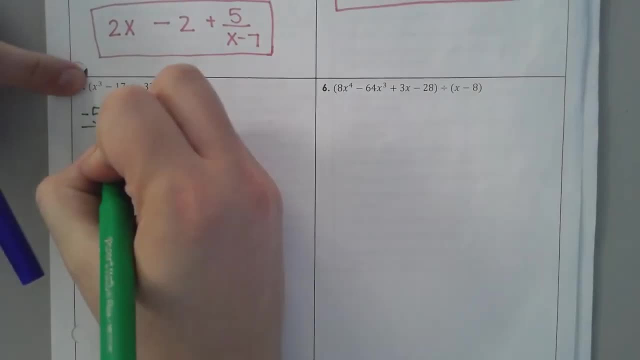 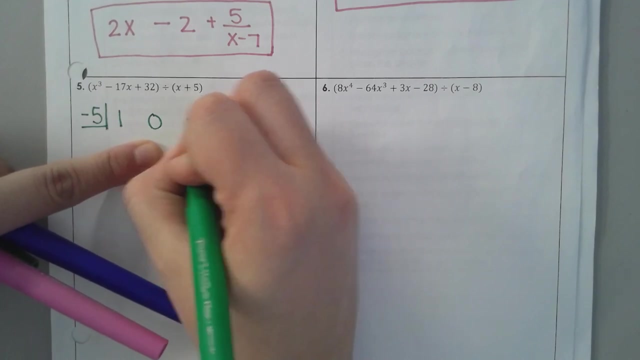 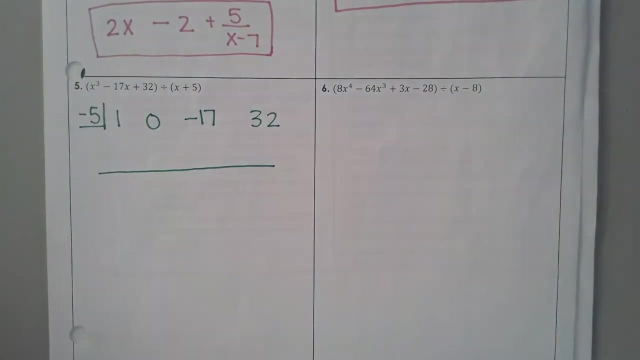 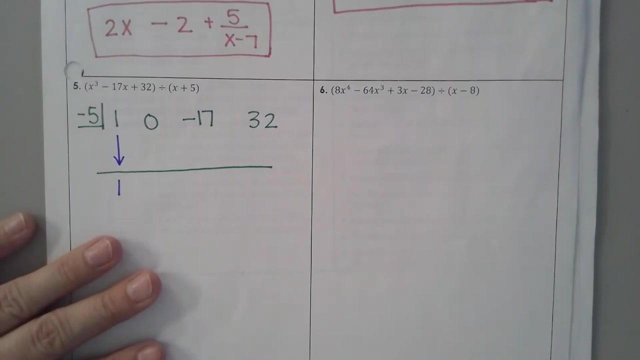 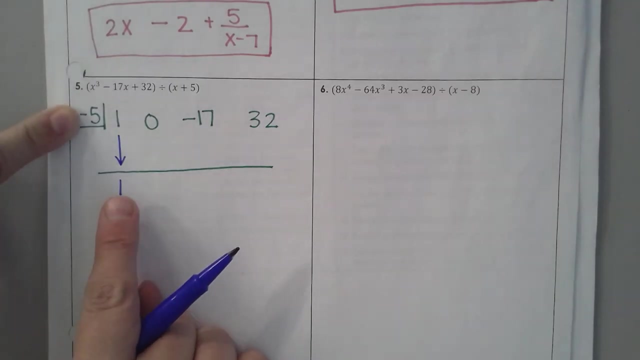 And then across the top, I'm going to have one zero, Because I have zero x squared, Negative 1732.. So you bring down your first number And then you multiply. What do I get when I multiply Negative five? 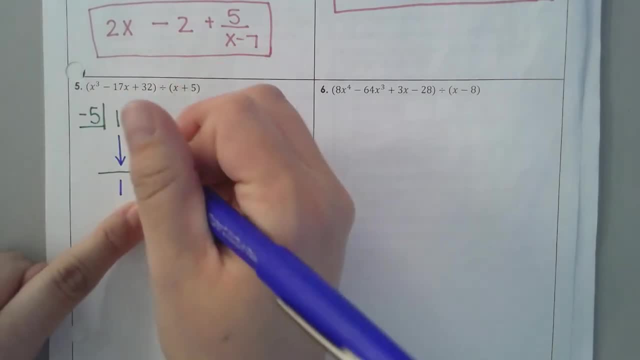 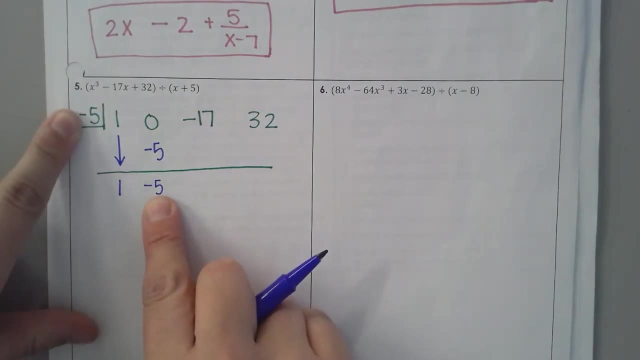 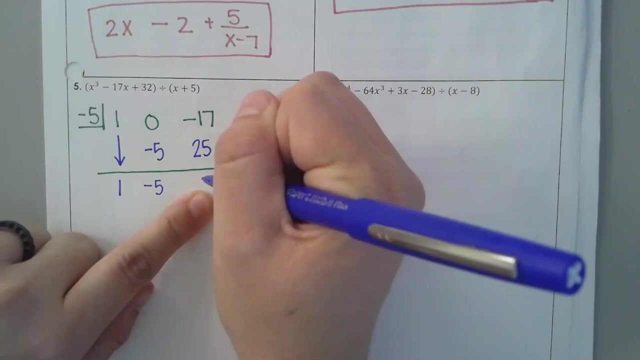 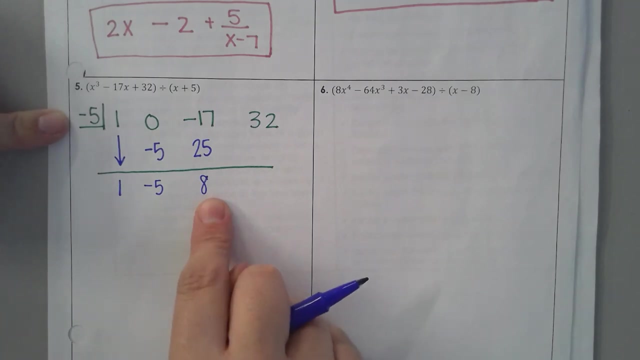 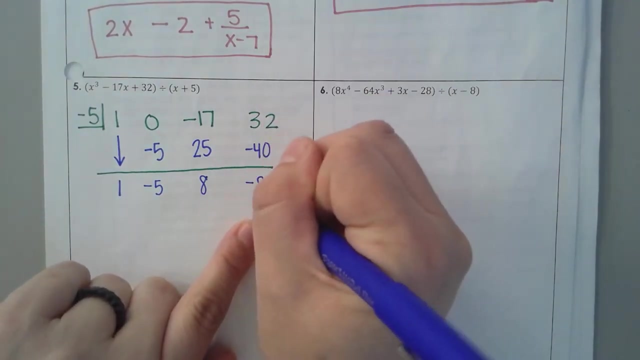 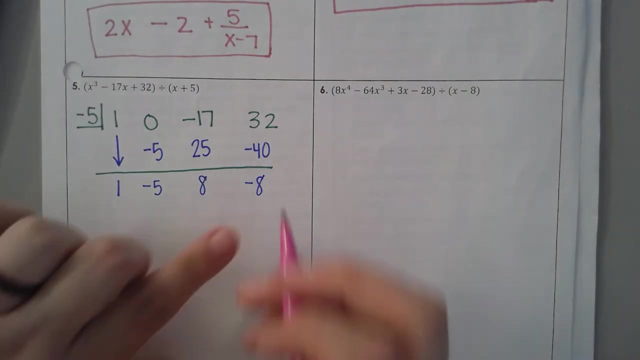 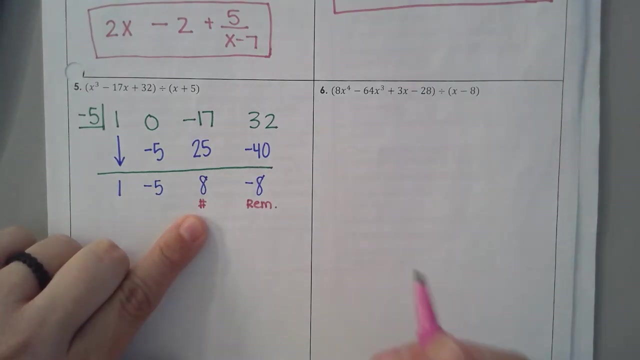 And then I add to get Negative five, Negative five. And then I multiply to get 25.. Add, I get what Eight, Multiply Negative 40. Add Negative eight: Good, So this is my remainder. this would be my constant, my plain number. 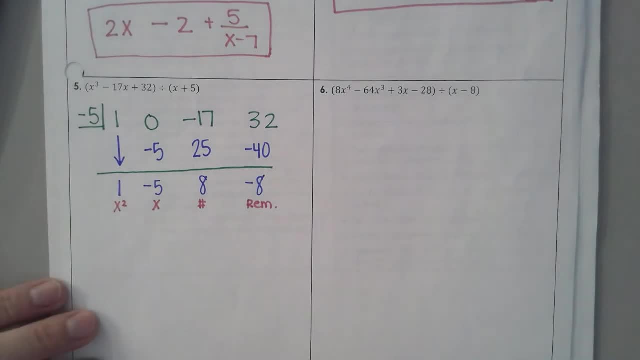 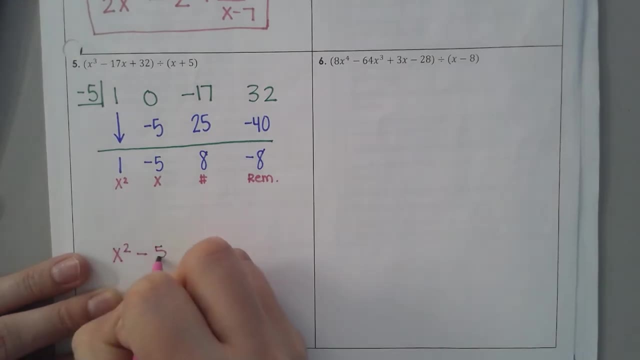 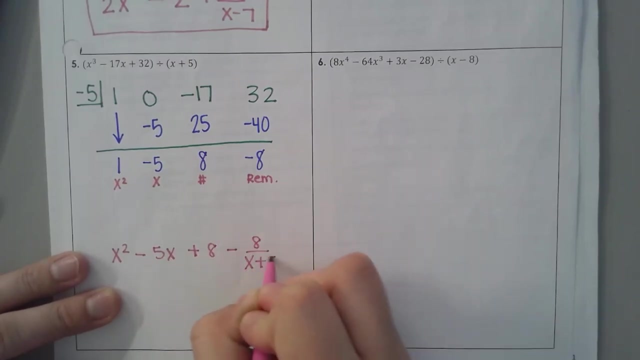 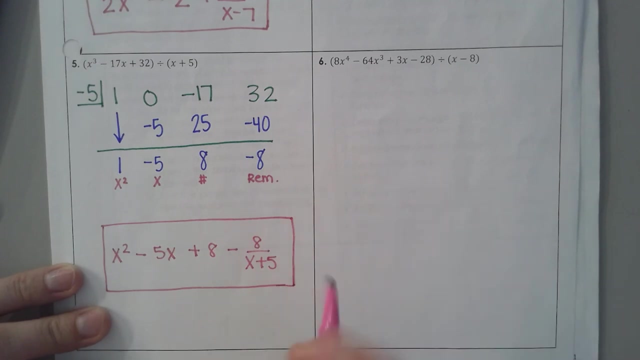 This would get an x and an x squared. So my answer is x squared minus five, x plus eight minus eight over x plus five. Then I have x squared plus x squared minus two, And then I add the result. I want you to try number six. 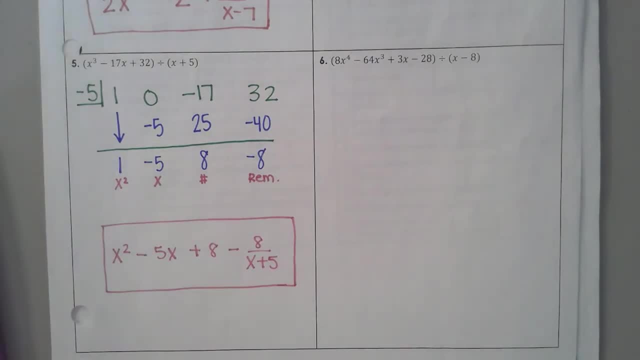 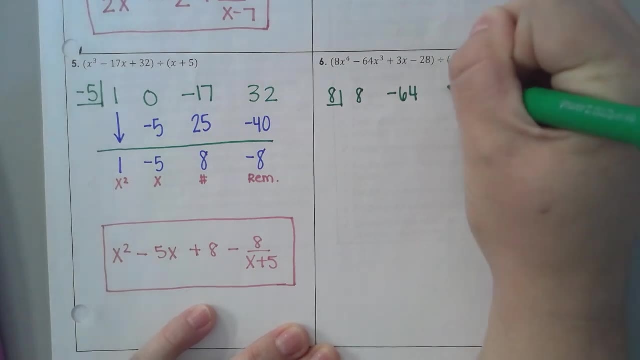 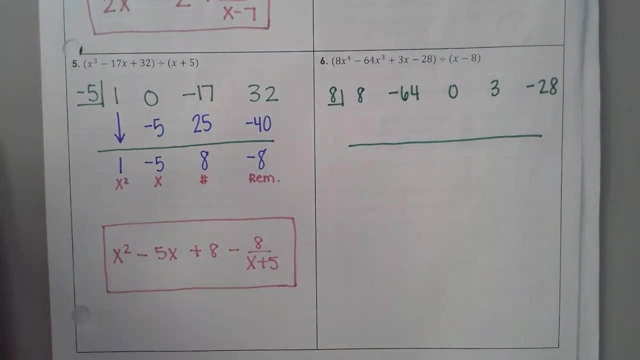 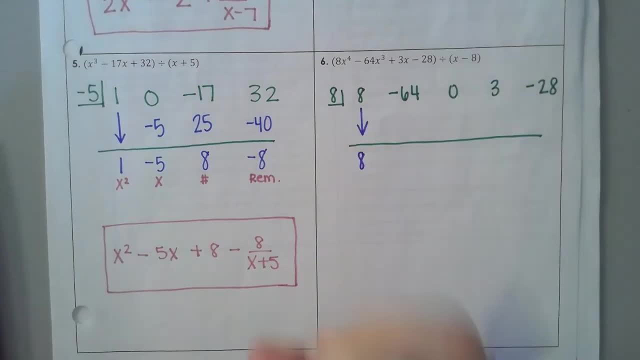 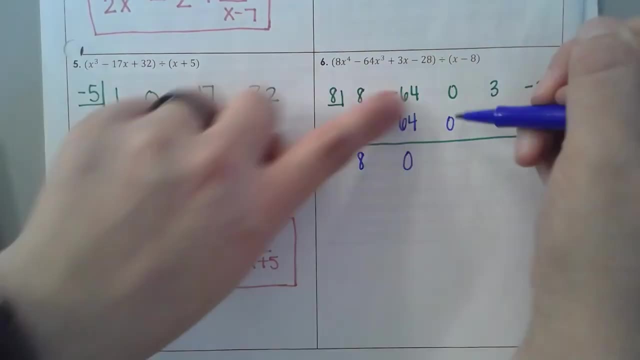 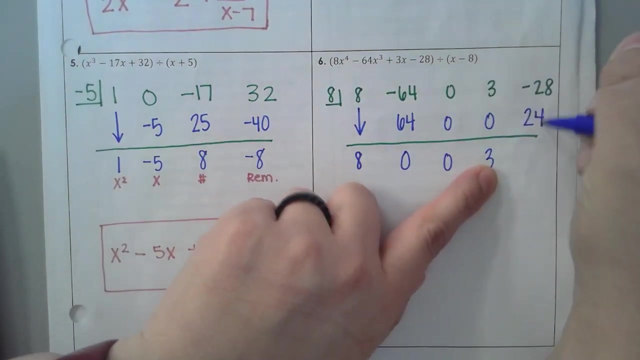 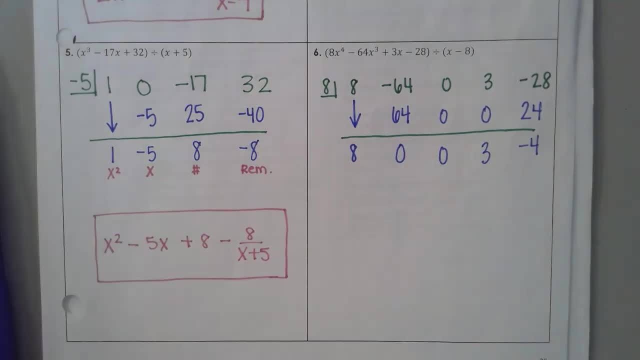 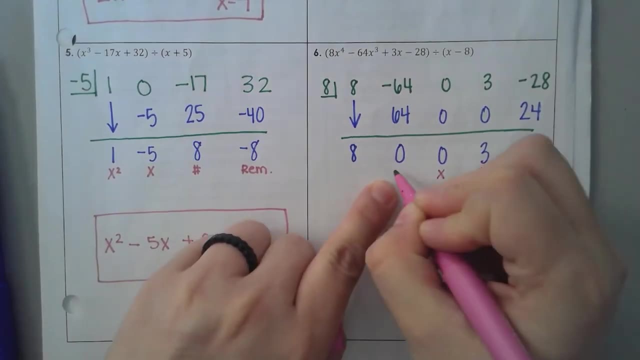 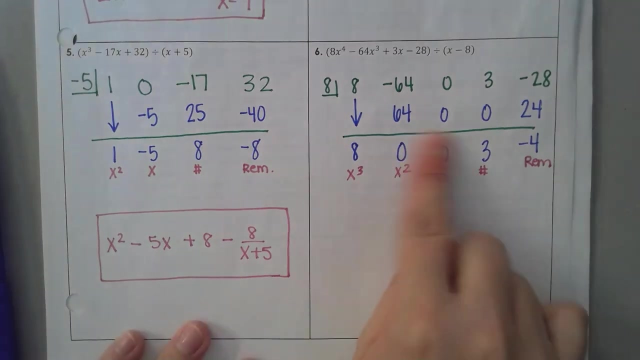 When this is the case, we're still going to label remainder number. This next one would be my: x, x squared, x cubed. We still label the same way, but when you write out your answer, you don't need to put the zeros. 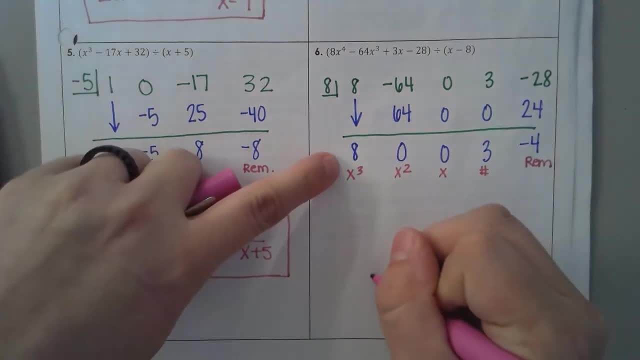 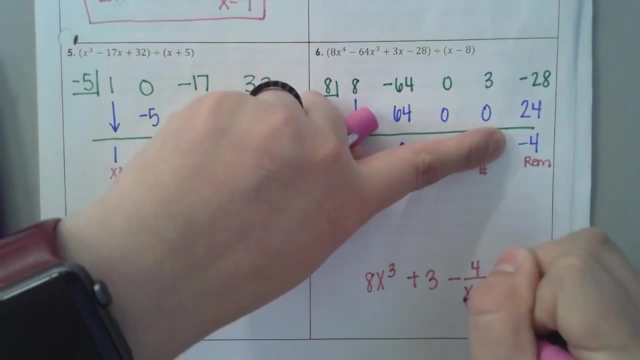 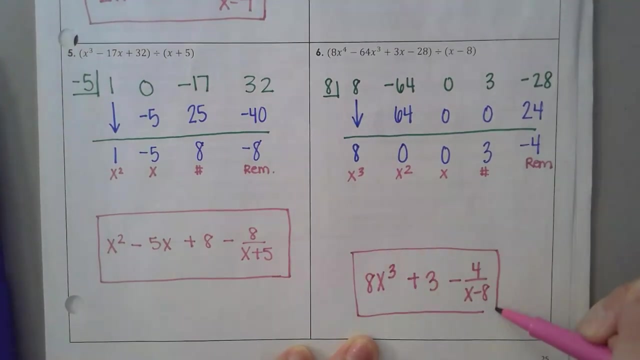 So my answer is 8x cubed plus 3 minus 4 over x minus 8.. Any questions?